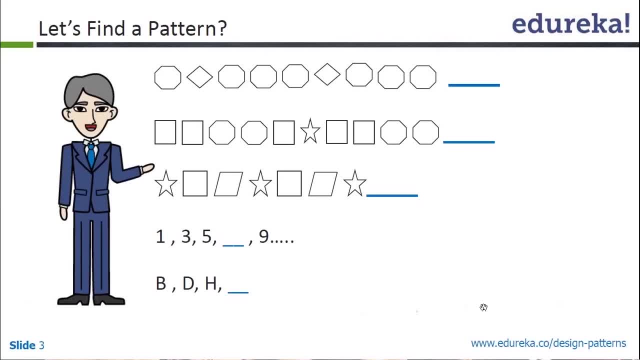 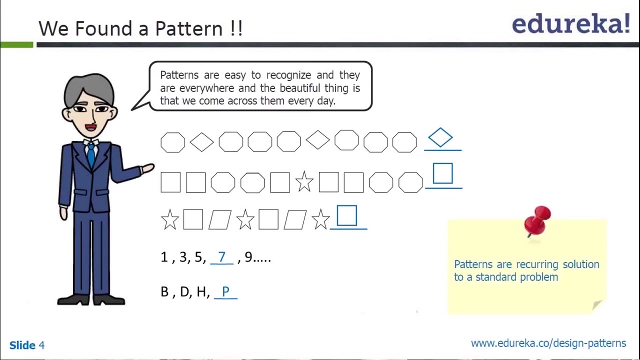 world of aptitude tests, and this is how, and therefore ability to figure out the pattern is a crucial one. Now, the pattern that we have on the screen here is the solution. One of the characteristics of the pattern are there are that they are easy to recognize, right, and we see them all the 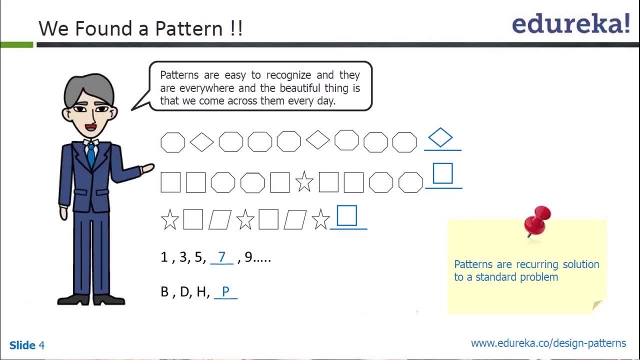 time. we just need to observe and you will see the patterns in the real life everywhere you look at it. and that's makes them very powerful, because they're observable, easily observable. the other people can also appreciate it and did use certain logic based on it. moreover, patterns come in handy because they are 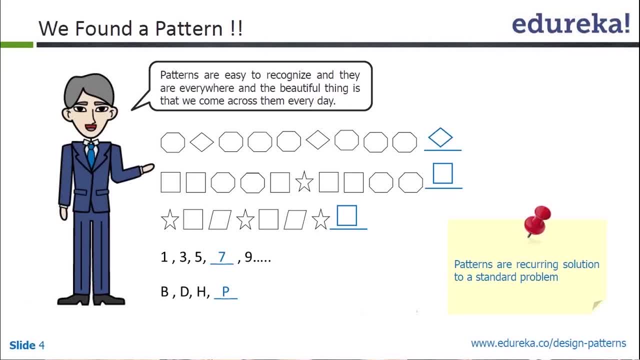 answers to some recurring problems, and because the problem is recurring, its best-known solution, that is, pattern, is also recurring. so you will see the yellow highlighted numbers are or diagrams are. the are the next in the sequence because we were trying to identify a pattern, since all of us 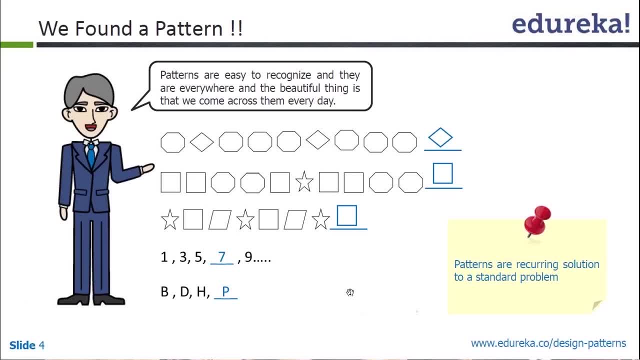 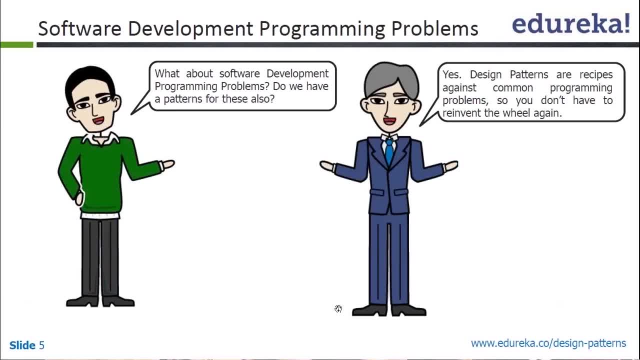 that's what you want as a algorithm. the parallel numbers are obvious, there are patterns always within with the of the models and the number of the patterns is always random. even at least 50% of half of the methods are not the same, but super obvious because game setters are exists in different programming. 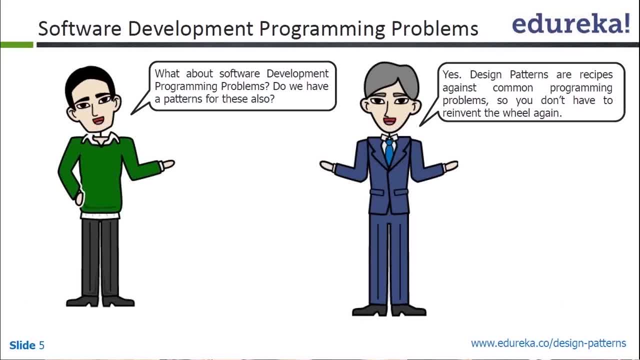 Because they are recurring solutions. they are very well understood by the industry And industry has also analyzed them for their weak points and the strong points, Where should we use them, or the context of the problem and the constraints. that is, what can we do or not do with those patterns? 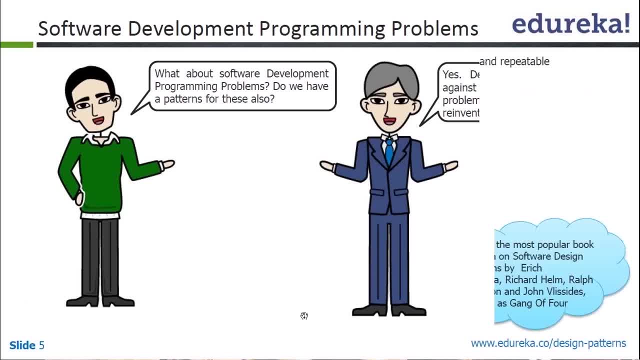 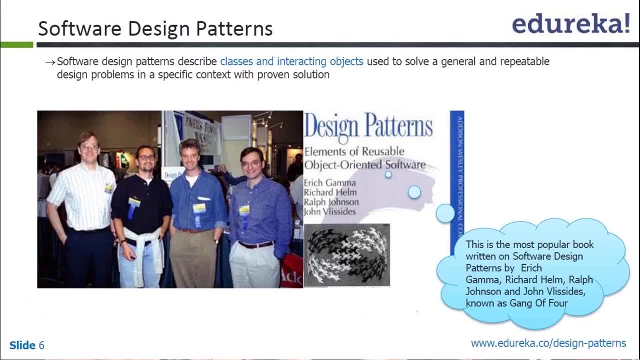 So here comes our pioneers in the space of design patterns. They are called Gang of Four and they were one of the first ones to catalog the design patterns. Now note this: These Gang of Four guys did not invent the patterns. They just analyzed the existing systems and draw commonality and they did not invent the patterns. 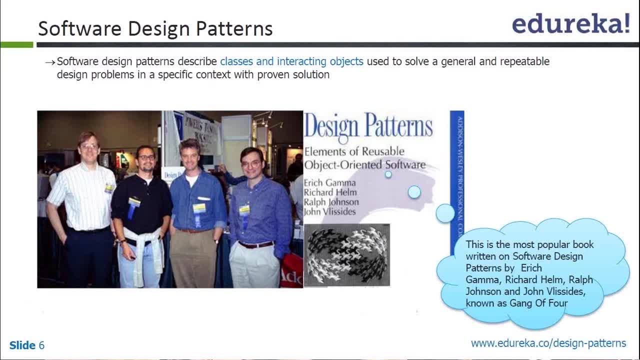 And cataloged them, that is, listed them as the design patterns. And it was a groundbreaking book, the one that they wrote, because it changed the way we think about software. and we then started saying, okay, so if we know the problem statement and if there is a match, we can very well pick up a design pattern from the catalog and solve the problem. 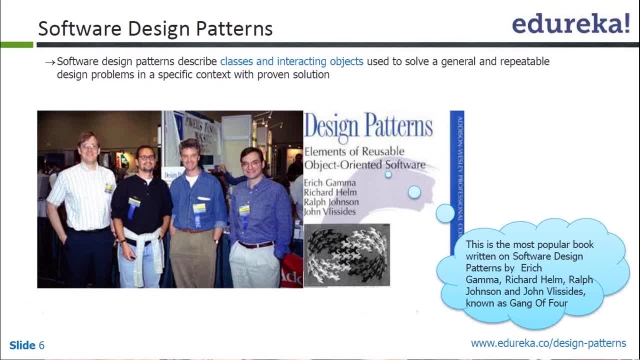 And we don't have to bang our head to figure out how do I solve it and all that. So we can also meet all the constraints and make it maintainable. So before I move on to the next slide, note their faces. how happy they seem to be. 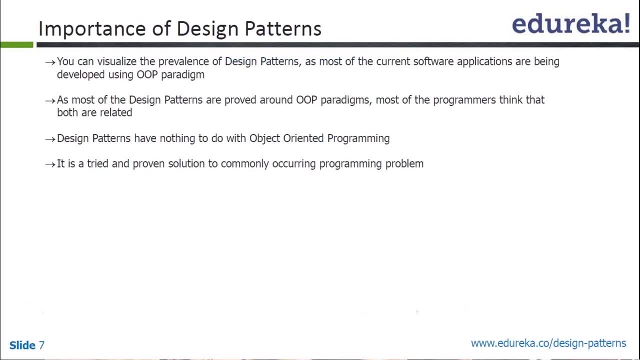 So importance of the design patterns. Well, one of the most important part in design patterns is industry experts understand them, and so can you and my peers, And it brings up a common language for people to talk to each other when they are talking about software development. 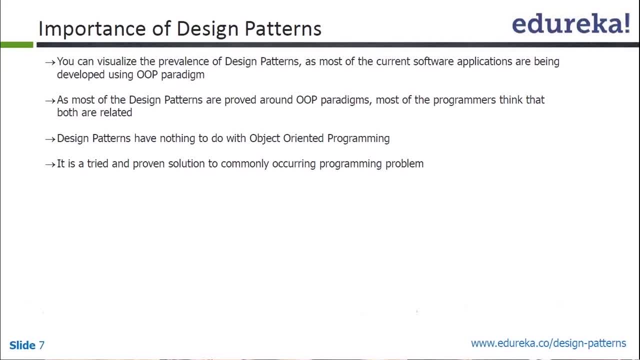 They also are based on, in recent time, something called object-oriented programming paradigm, which is the most popular methodology of developing the software. But it also comes with a downside. A downside is that many programmers, and sometimes engineers, their designer, falsely assume that design patterns and object oriented paradigms 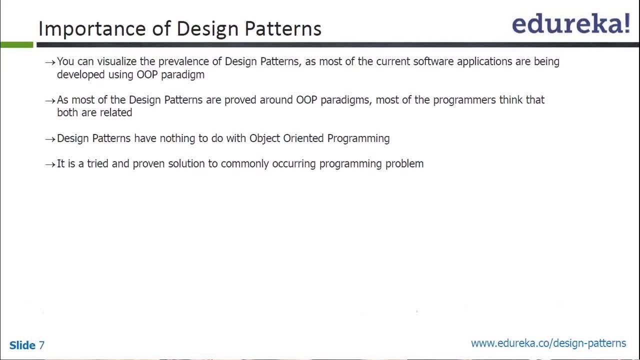 are one and the same, but they are not in general patterns. and then design patterns are nothing to do with a specific kind of programming paradigm, in this case object oriented, because object oriented is more prevalent. therefore, the design patterns for object oriented world are more prevalent. most importantly, these design patterns are tried and proven solutions to 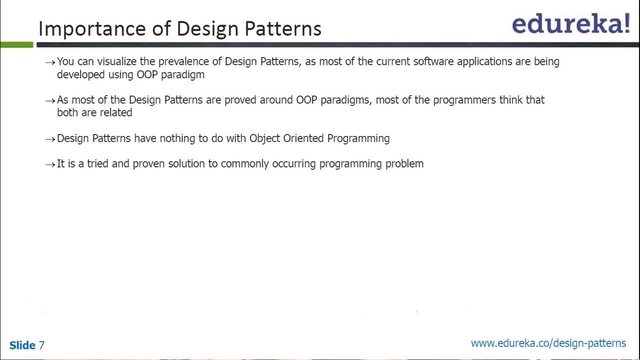 programming problems, the problems that recur, and if we choose to implement a particular design pattern to solve a particular problem, it guarantees us that the next person who is going to maintain the code understand it, because they will be able to understand the design pattern and we also know the weaknesses and strengths of those design patterns. so 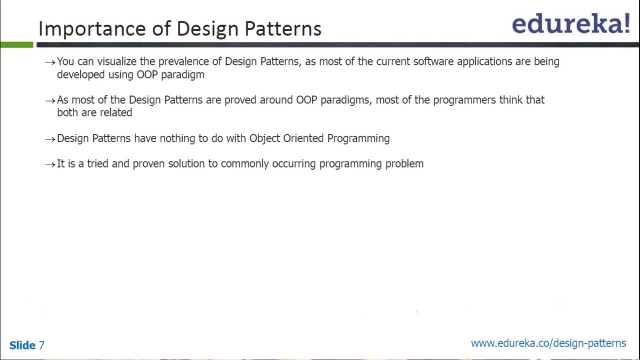 should the context change? we will be really looking at the design pattern and say whether it is still okay to use or should we switch it toward or swap it out in favor of another design pattern. today we are going to look at a use case, a problem statement. we're gonna say that. 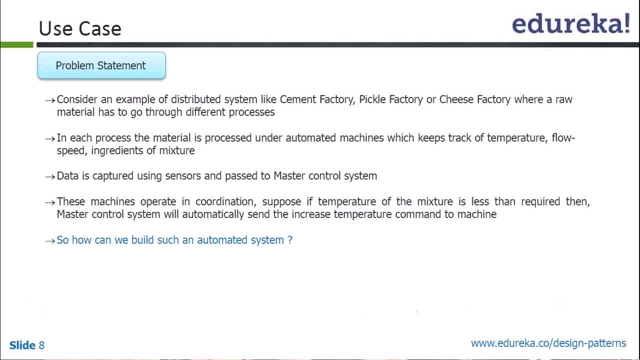 let's, let's there, let there be some sort of factory, a factory which which consumes the raw material and produces the finished good. that factory could be a cement factory, or a pickle factory, or a cheese factory, even a chocolate factory, if you like. the factory is going to get some material, some raw material. there would be some. 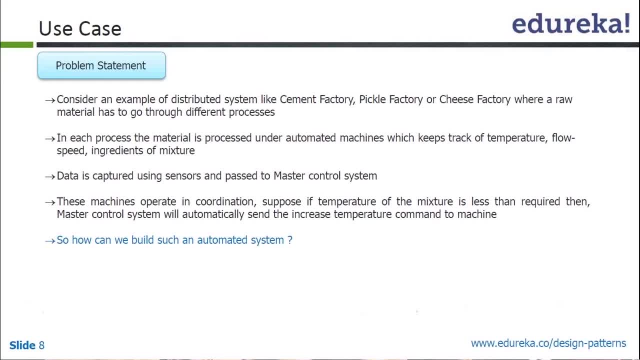 automated machines that keep track of the speed, the temperature, the ingredients and all and the data captured we use. the data is captured using sensors, various sensors employed in this automated system, and these sensors are going to send their input to the master control system. the master control system will look at those sensor values and operate on the data that 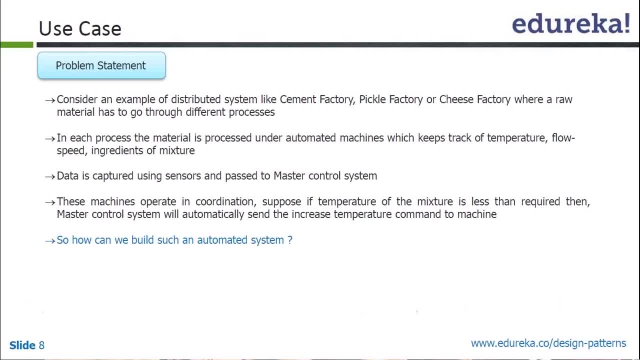 operate on the data, decide what action to take, and then action is relayed to something called actuators which may change the temperature and may change the mixture proportion. these machines operate in coordination. if one of the part fails, the the operation is kind of cannot be completed, so there needs to be. 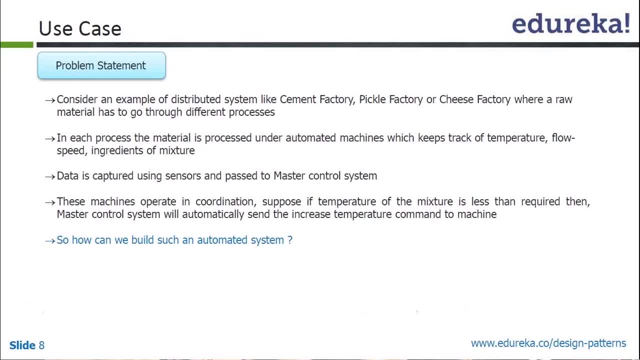 communication between these entities in your factory, for example, a temperature sensor talking to the master controller and master controller talking to, maybe, a furnace, an electric furnace, to either lower the temperature or increase the temperature. a real world scenario question will be: how can we build this automated system? 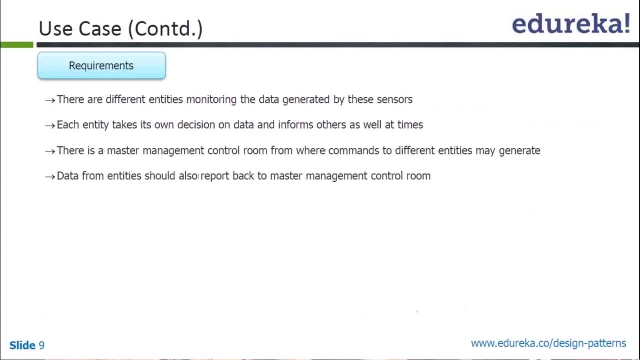 so we'll continue with this use case and requirements. we are saying that let there be different entities that are monitoring data generated by the sensors. each entity can take its own decision on data, as well as inform to other. for example, a temperature sensor may display it to a human operator as. 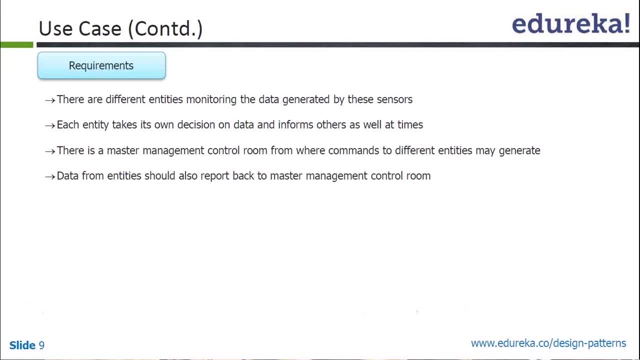 well as send that data to the master controller, and there is a master management control room where the commands for two different entities are generated, which is solely responsible for the good and safe operations, and the data from the entities is also sent back to the master management control room where it is processed and actions can be taken in. 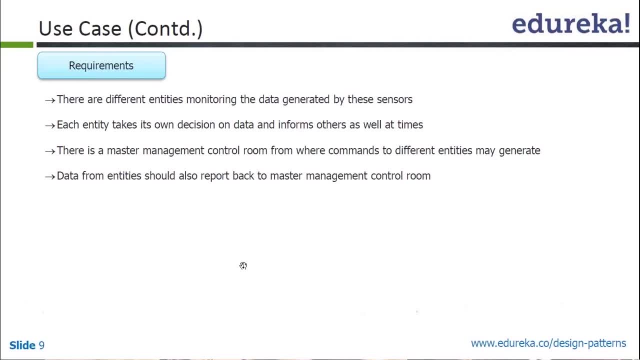 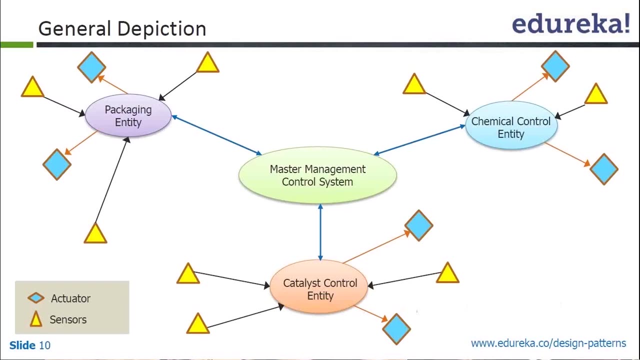 some cases even the audit logs can be generated with that. moving on, here is the general depiction of the solution would look like there could be packaging entities, the master management control, the catalyst control and the chemical control entity. and you see these blue diamond, they are actuators. so all these bubbles are gonna. 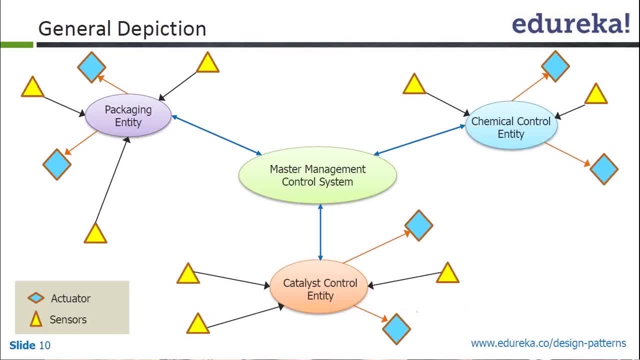 operate on actuators and there's yellow rectangles are are sensors. who are gonna send data to these bubbles? if you look at it, the master management control is a central entity which is responsible for the operation of this factory. there are three other entities which are separate domains, some 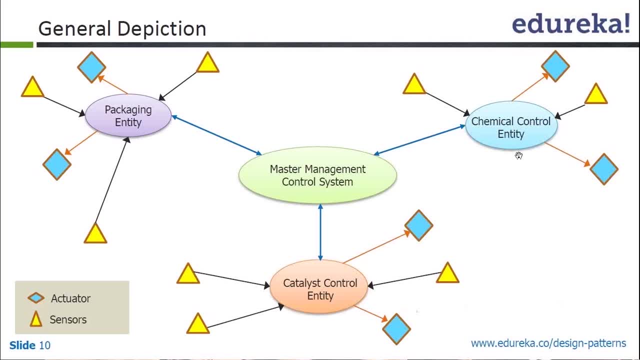 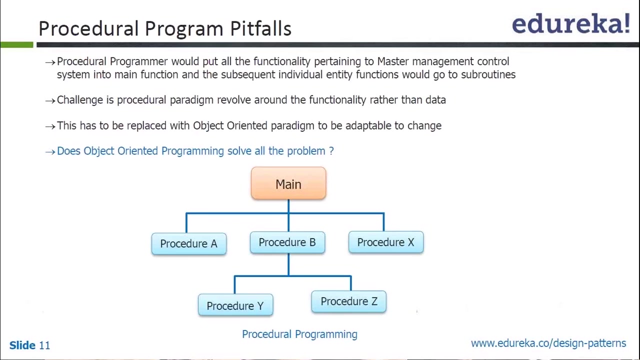 handling, chemical composition, catalysts and packaging. but it is the master management controller system which orchestrates various operations in this. so this is gonna be a general depiction. we will then come to how a non object oriented world can program it. they will probably go by procedural system and they'll put all the functionality pertaining to management control into something called the main function, and then main function may have certain Themей y, all the functional. 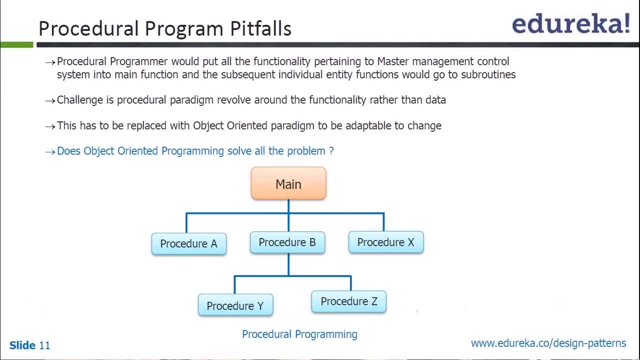 helping procedures or child procedures, subroutines which allow main to segment. it works well. it may solve your problem but it may be hard to maintain what happens. for example, the catalyst composition needs to change. you'll have to figure out the exact procedure where it needs to change. go update that. 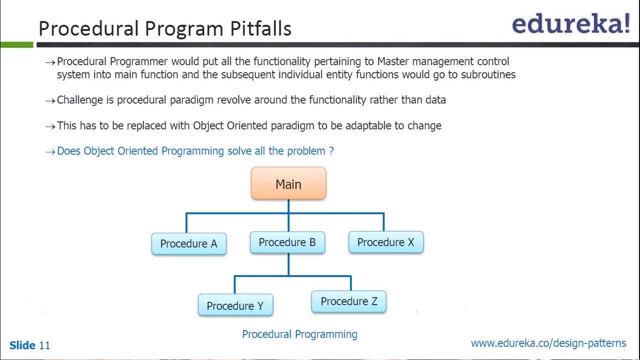 procedure, recompile your code, test it out and then deploy it into a production system. now the the challenge here of the procedural system is that it thinks like human brain. you know I walk up the stairs. if I need to go to, let's say, a third floor, I know that I have to walk up to the base of the staircase or at 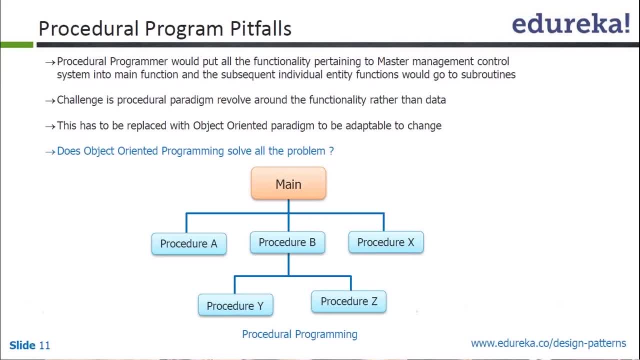 elevator area and do a next step: maybe start climbing or requesting the elevator, based on what we choose to do, and so on and so forth. essentially, a procedural language is more like one looking it from a single point of view. in this case, if a human needs to go to third floor, human 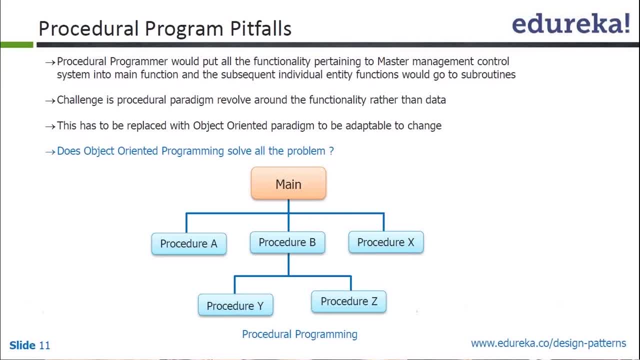 will start thinking what he needs to do and not what an environment, what needs to happen in the environment that he is living in. such procedures would be good if you are building a very small application, maybe something that accepts the data in the single form in a web UI, but this cannot scale when we are. 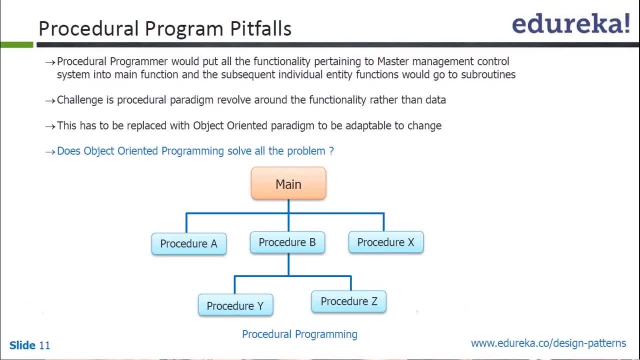 talking about complex enterprise-wide applications, especially those applications who are to be, which are to be maintained for, let's say, five to seven years. in fact, what ends up happening if you write procedural programming there is you write a lot of spaghetti code and episode above and therefore, in general, one would want to move into the 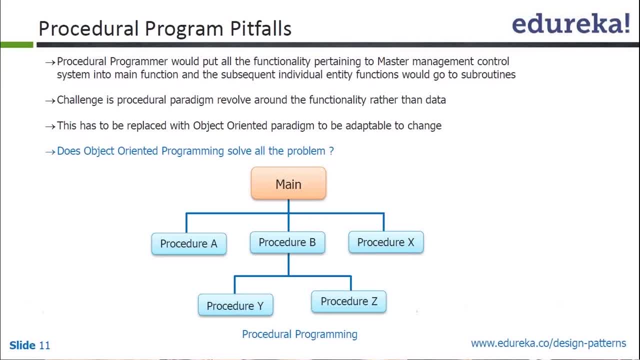 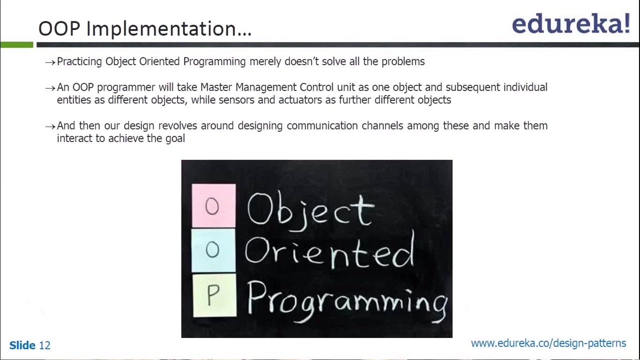 object-oriented paradigm, where each entity is represented by an object or a set of object, and that allows you to maintain the program in the long run. here comes the object-oriented world's kind of introduction. with any technology it's not gonna solve all your problems, or I'm're not gonna forget to tell you that. 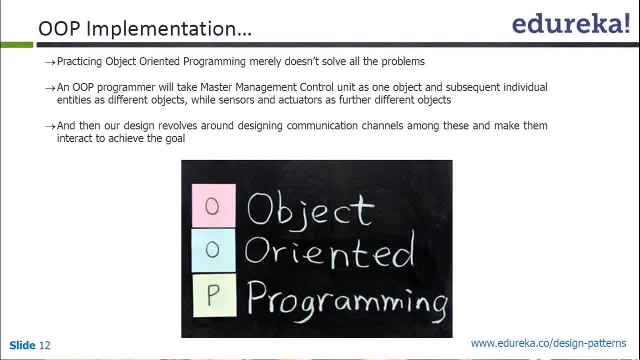 because the way the device is needed to FLST is the average fb inteen 7x20, Savage slide problem extremely 550 for images and other methods of grid design worlds kind of introduction that any technology it's not gonna solve all anything problems just by using it. one has to be a little more intelligent as to find out. 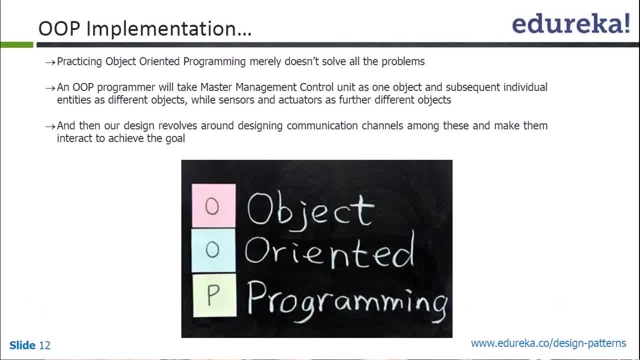 how to to use it. there is an old saying which goes like: the one who has a hammer thinks that every problem or everything is a null. we will be doing good if we remember that we don't own a hammer. and if we own a hammer, not every problem is. 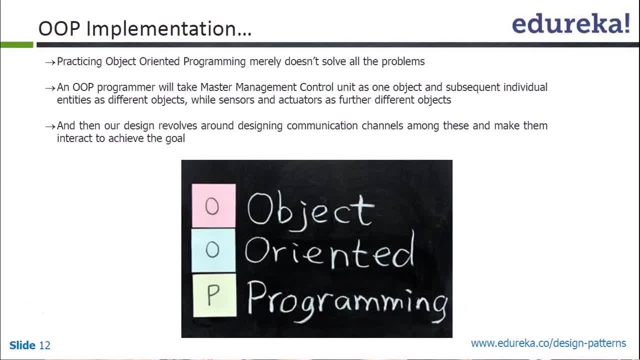 a Nell, you don't have to use the same old stuff to solve any new problem. then what problem should we be solving by having that hammer or, in this case, having some known solutions? that's where need of understanding design pattern comes in. so talking little, let's talk a little bit about object oriented on the 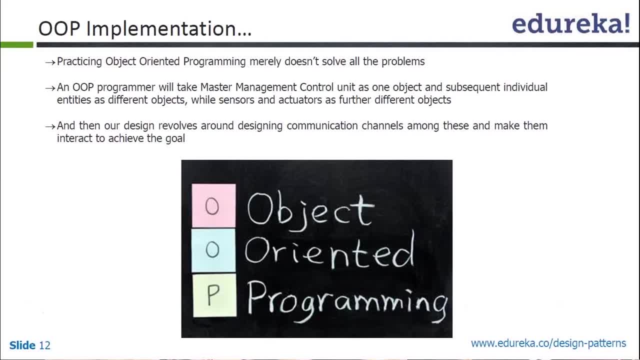 slide. an object oriented programmer may take a master, control, manager, management control unit in a one object and subsequently. different entities are different objects and you one would want them to talk to each other to achieve certain use case. so, as rightly noted there, once we have identified the objects, the only remaining part is to find out how they 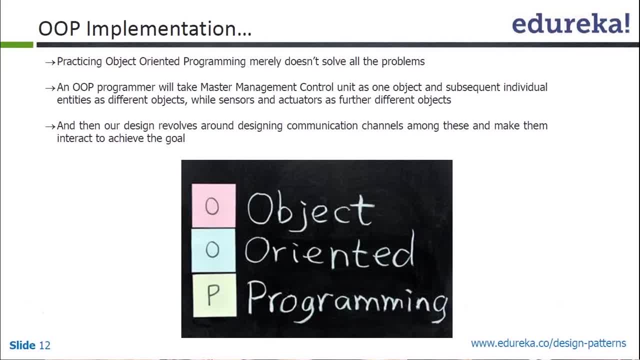 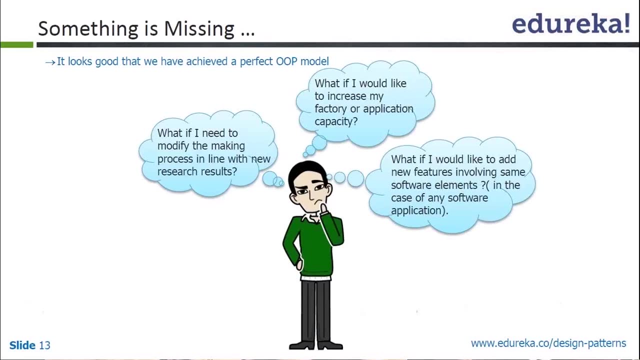 will talk to each other, communicate to each other and to to achieve a same common goal, in this case, the use case that we talked about. when we look at it, we definitely know that there is something missing. and what is? what is it missing? well, how about? a change required because 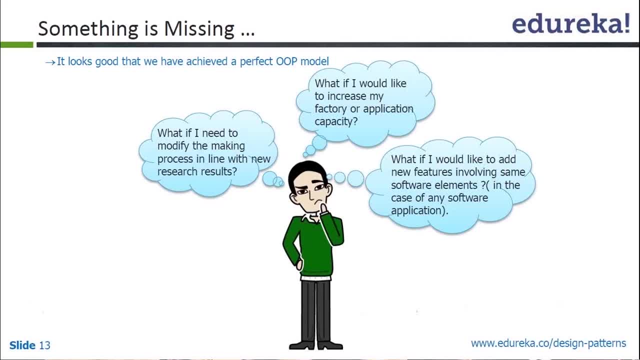 there is a new research coming in, or how about I want to scale up my application? in this case, for example, I want to increase the unit production per day of my factory. in the software world, that will mean: how can I make my application run faster? and, most importantly, which is the 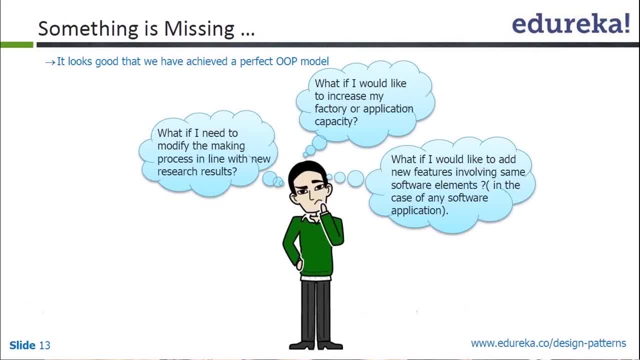 life of any software. it has to evolve because the business needs change and sometimes we add functions or features to the existing existing software. let's say, in case of a cement factory, I want to change my packaging from a 50 kg bag to maybe a 10 kg bag, or, and I also want to- 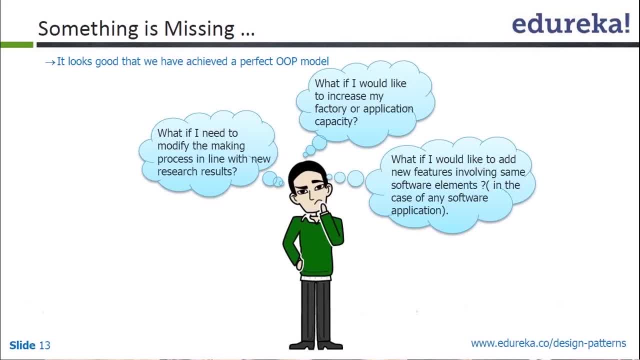 let's say, change the material of the sack in which my cement gets packaged in. so in the in the life of a software, it is important to understand initially that a code needs to be maintainable. if I may share with you some statistics, it is very likely that the programs of this teams Forgive me for using here any healthcarelıkThanks you for your support. 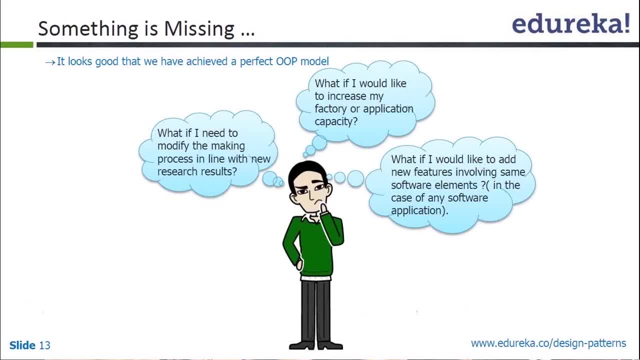 likely that a software application will spend 80 percent of its life time in the maintenance mode, where you know you're just making sure that the software survives in the production. perhaps we spend about 10 to 12 percent of the time designing a system and only maybe eight percent time to write the code and test the code. 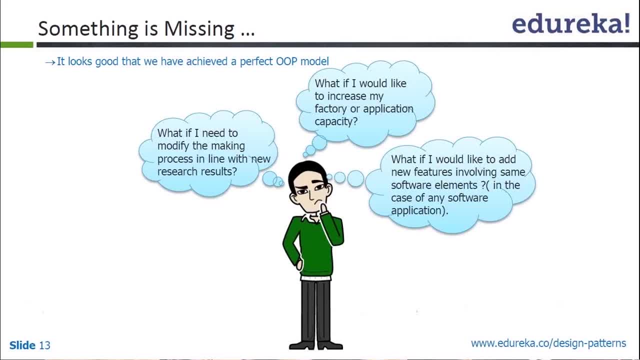 and therefore, while building any system, one has to also consider: what does it take to maintain it? and that is where, if you know the design patterns and if you apply them correctly, the answers will come naturally. every design pattern will have, as i said, its own strength and weakness. and what? 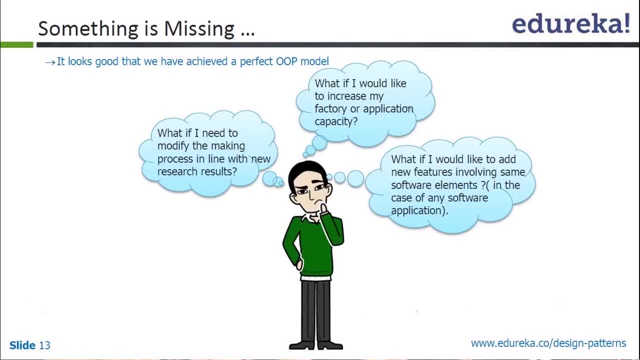 matters in the maintenance mode of a software is: how do we cope up with the weakness of any system? so, as i said, the design patterns are are kind of catalogued right, and if you know the design pattern and if you know how to use it, you would be a better software developer. but there's a 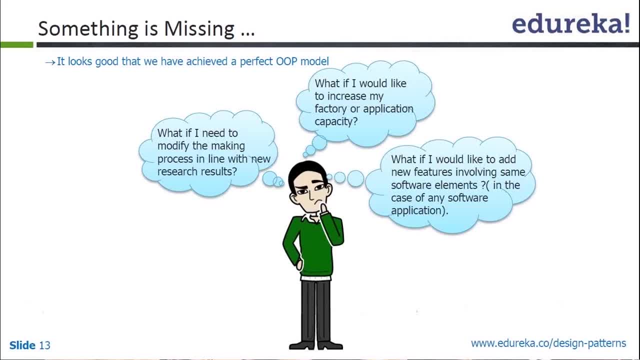 difference between knowing what a pattern is and knowing how and when to use it. if i may draw your attention to a difference between a knowledge and a wisdom. a knowledge will say: oh, there is a design pattern catalog wherein there are patterns xyz and it is to be applied in certain cases. 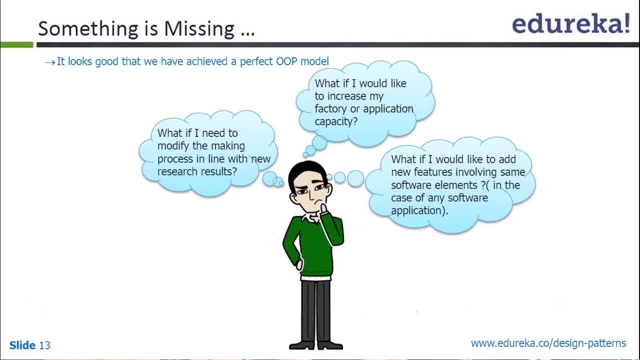 but it is a wisdom which will tell you when exactly to use it, when, when you should not be using it and generally. that comes with experience and i'm here with you to share that experience and some sort of wisdom. there is an old saying, if i may quote it here: knowledge is like knowing. 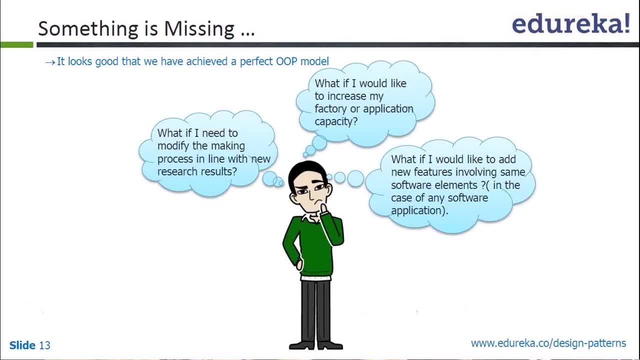 that tomato is a fruit, but wisdom is knowing that it is not to be put into a fruit salad. so if you look at a design pattern catalog and you find out, oh well, there is an abstract factory, but if you don't know when and how to use it, that knowledge is not really, not really. 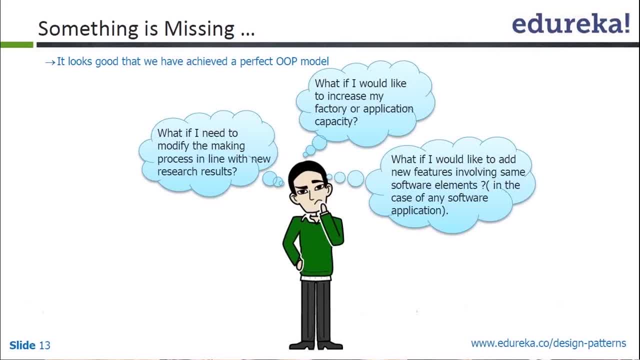 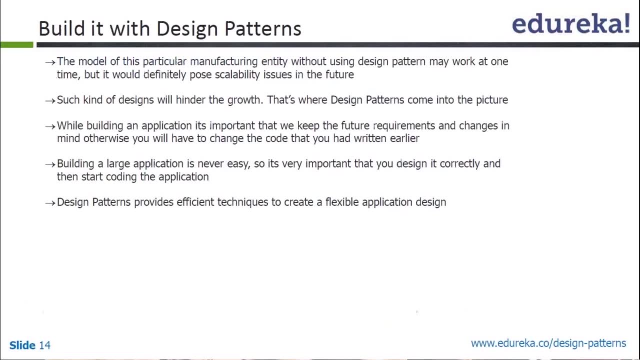 useful, isn't it? you'll probably be creating more mess than you started with, and that's where we come in. we want to share with you the experience that we have in industry and knowing, for example, an abstract factory: what is it and how to use it, and what is the consequence of. 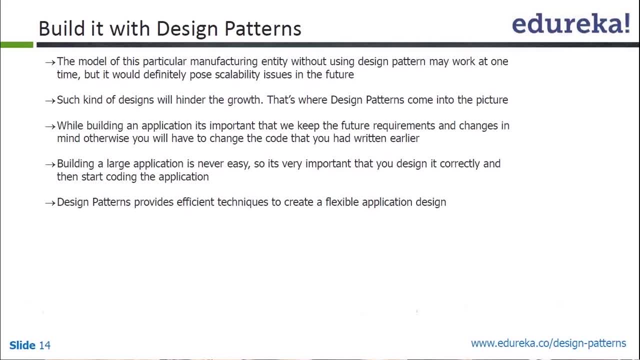 using it in the maintenance mode. so with that, i am moving to the next slide. uh, we're saying that we will model this manufacturing entity, uh, with some design patterns, for example. if you don't do it with design pattern, it will work, but then in future, when you want to extend the 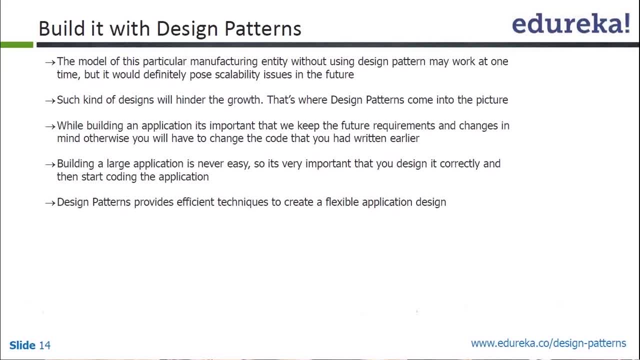 functionality or make it more maintainable or scalable. it will be a hard task to take up. see the so one i also have to understand. um, okay, most of the time we think about building a new software. have we thought about when the software dies? well, i can tell you. 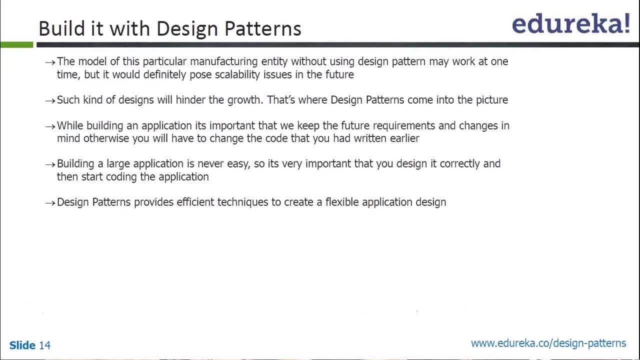 that the software dies, meaning the software is taken out of production when it is no longer economical to maintain it. the code has become something called a spaghetti code. the original developers who developed it are no longer with that organization and they, the new developers, did not perhaps got the entire kt, or did get the kt, but did not get their facts together. 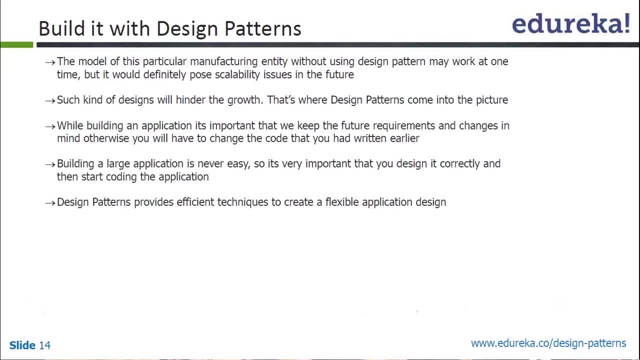 and it is cost prohibitive to add feature to that software. in such cases the architects and the business stakeholders will want to think about building a brand new system. and if the brand new system is not developed well, the cycle repeats. very soon the software will age it. it is not beneficial to maintain or it is a cost prohibitive to maintain that system in. 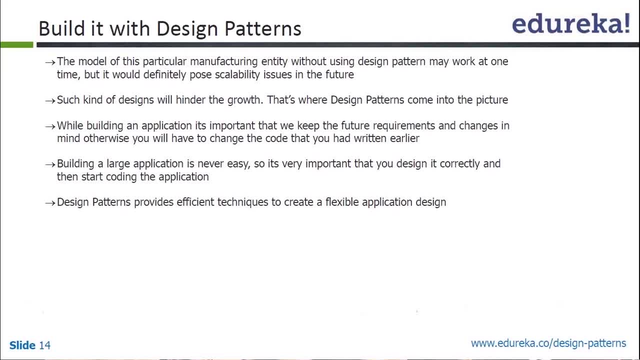 production, and then architects and business stakeholder holders will come and say, oh, they want to build a new system. so using the right solution- in this case, right design patterns- extends the life of the system, and that's where it is important for us to know the design patterns and know how to use it, not 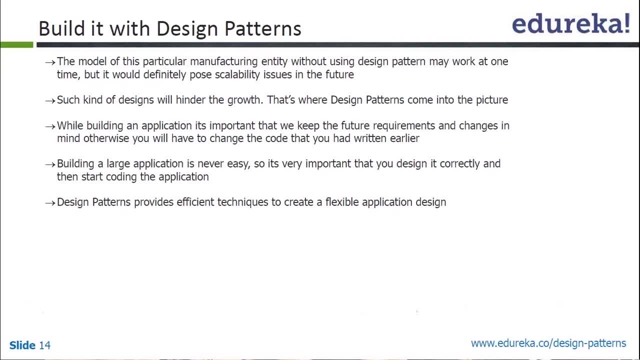 only for the fresh or green field projects, but also for the projects under maintenance. design patterns are generally a common language between the development organizations for a lot of people. So if you are building a factory pattern, for example, if you are building an abstract factory pattern somewhere in the comments, you will say that well, this is a standard abstract factory pattern. 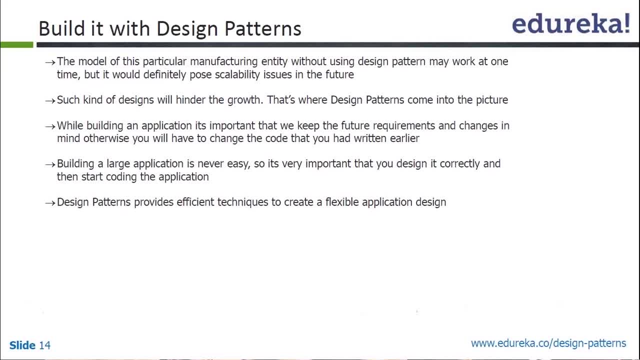 and let's say three years, four years down the line, somebody wants to come in and in the maintenance mode, enhance it or kind of make some changes because of maybe a business scenario changing. the person will read abstract factory pattern. he'll easily be able to correlate the related classes to those uh entities in the abstract factory or any other. 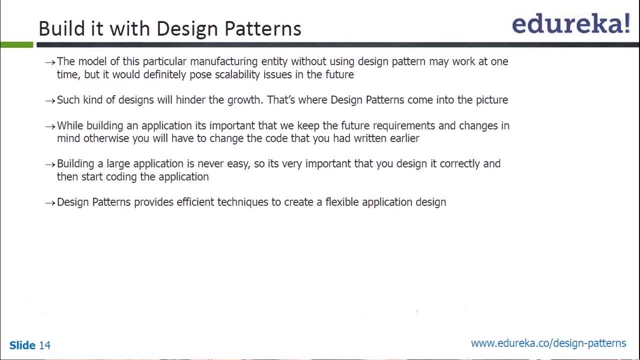 pattern, for that matter. right, that makes it very maintenance of a large enterprise scale applications moderately easy to maintain. um now they are because design patterns are proven solution. you also know the consequences. should there be a man in the maintenance mode, should there be a uh added requirement um to a scenario which makes that design pattern not so lucrative, one will have.